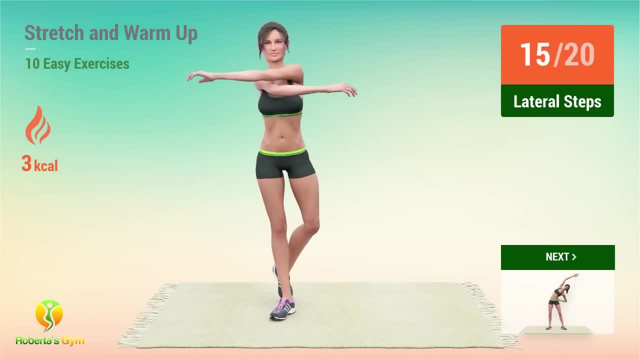 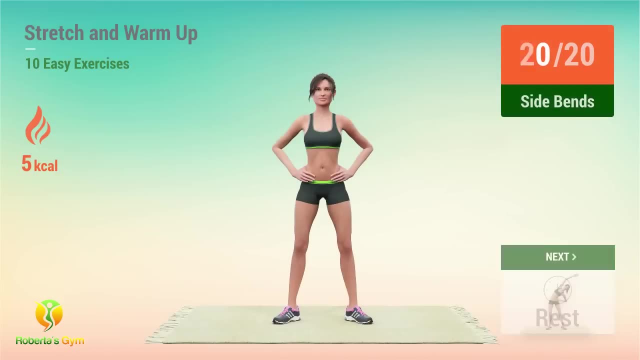 14,, 15,, 16,, 17,, 18,, 19,, 20.. Up next side bends In: 5,, 4,, 3,, 2, 1, go 1,, 2,, 3,, 4,. 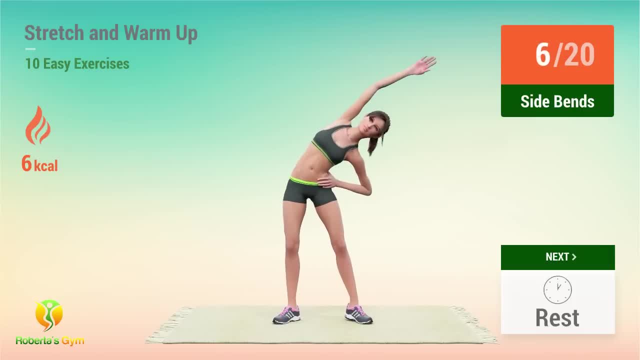 5,, 6,, 7,, 8,, 9,, 10,, 11,, 12,, 13,, 14,, 15,, 16,, 18,, 19, 20.. 5,, 6,, 7,, 8,, 9,, 10,, 11,, 12,, 13,, 14,, 15,, 16,, 17,, 18,, 19, 20.. 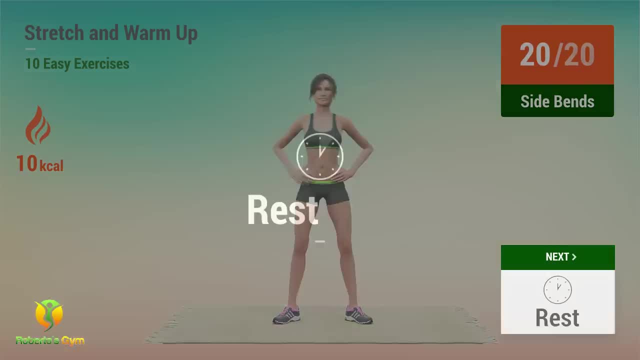 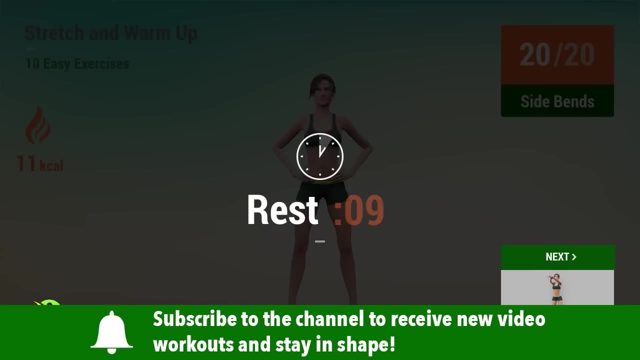 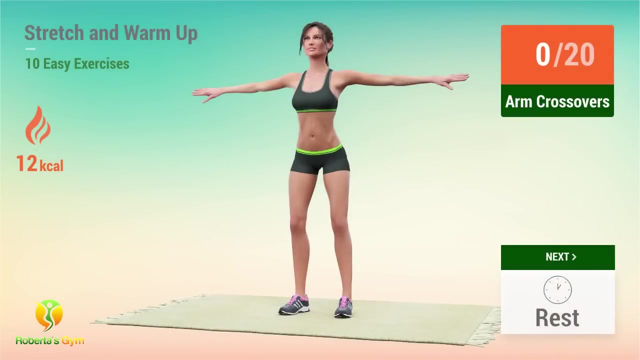 19, 20, rest time Up next arm crossovers In 5,, 4,, 3,, 2, 1, go 1, 2,, 3,, 4,, 5,, 6,, 7,, 8,, 9,, 10,, 11,, 12,, 13,, 14,, 15,, 16,, 17,, 18,, 19,, 20.. 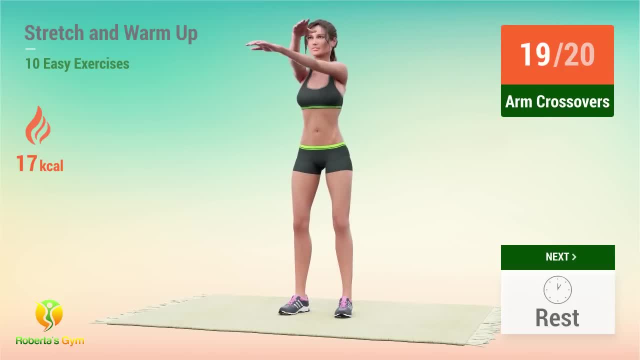 In 5,, 4,, 3,, 2,, 1, go 1, 2,, 3,, 4,, 5,, 6,, 7,, 8,, 9,, 10,, 11,, 12,, 13,, 14,, 15,, 18,, 19, 20.. 1,, 2,, 3,, 4,, 5,, 6,, 7,, 8,, 9,, 10,, 11,, 12,, 13,, 18,, 19, 20.. Rest time. 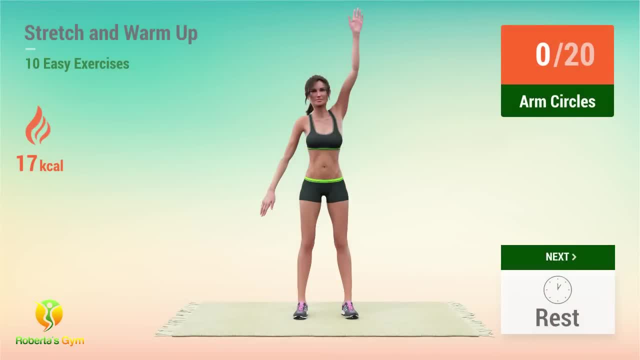 Up next circle squats In 5,, 4,, 3,, 2,, 1, go 1,, 2,, 3,, 4,, 5,, 6,, 7,, 8,, 9,, 10,, 11,, 12,, 13,, 14,, 15,, 16,, 17,, 18,, 19, 20. 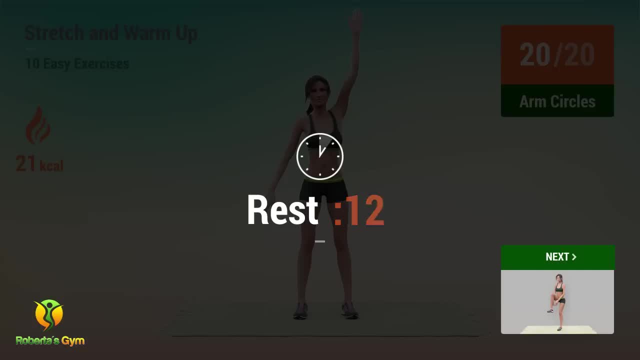 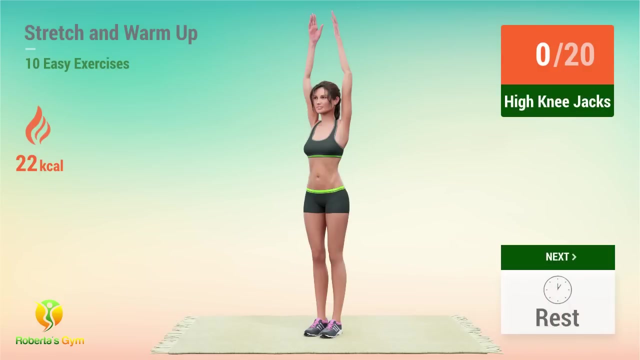 Rest time. Up next High Knee Jacks In 5,, 4,, 3,, 2, 1, go 1, 2,, 3,, 3,, 4,, 5,, 6,, 7,, 8,, 9,, 10,, 11,, 12,, 13,, 14,, 15,, 16,, 17,, 18,, 19, 20. 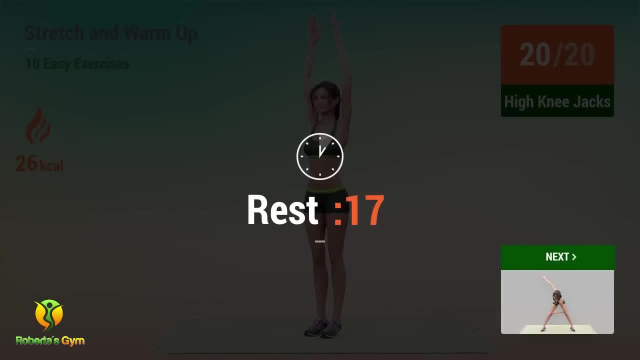 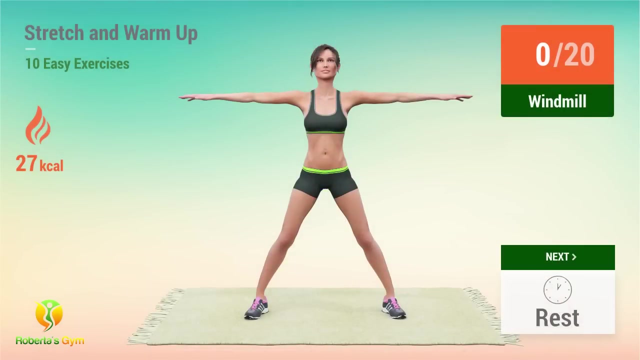 Rest time. Up next Windmill In 5,, 4,, 3,, 2,, 1, go 1,, 2,, 3,, 4,, 5,, 6,, 7,, 8,, 9,, 10,, 11,, 12,, 13,, 14,, 15,, 16,, 17,, 18,, 19,, 20. 1,, 2,, 3, 4, 3, 4,, 5,, 6,, 7,, 8,, 9,, 10,, 11,, 12,, 13,, 18,, 19,, 20. 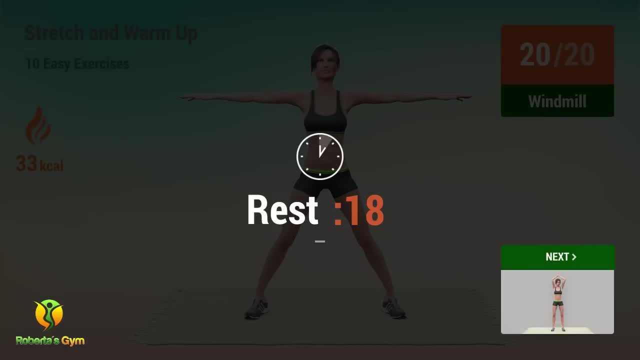 Rest time: 1,, 2,, 3,, 4,, 5,, 6,, 7,, 8,, 9,, 10,, 11,, 12,, 13,, 14,, 15,, 16,, 17,, 18,, 19, 20. 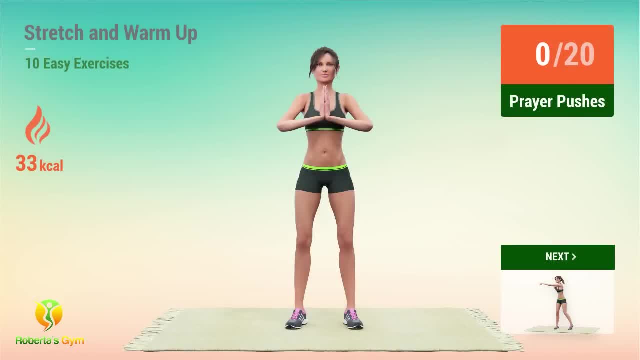 Up next Prayer. Pushes Up next Prayer. Pushes In: 5,, 4,, 3,, 2,, 1, go 1,, 2,, 3,, 4,, 5,, 6,, 7,, 8,, 9,, 10,, 11,, 12,, 13,, 18,, 19,, 20,, 20. 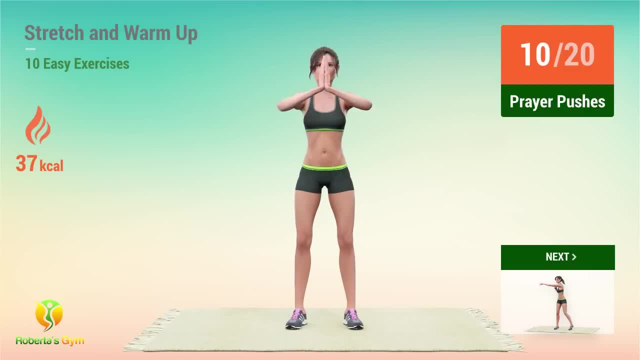 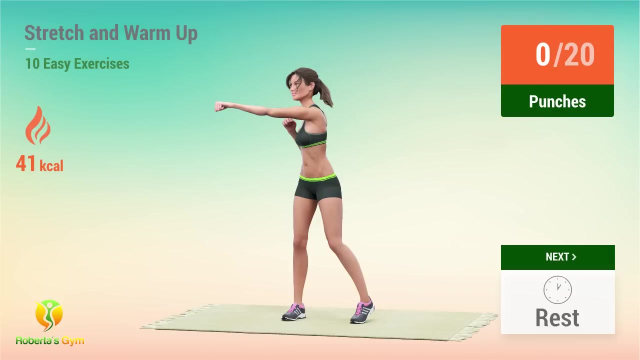 Rest time Up next Windmill: Ten, Eleven, Twelve, Thirteen, Fourteen, Fifteen, Sixteen, Seventeen, Eighteen, Nineteen, Twenty. Up next punches In five, four, three, two. one go One, Two, Three, Four, Five. 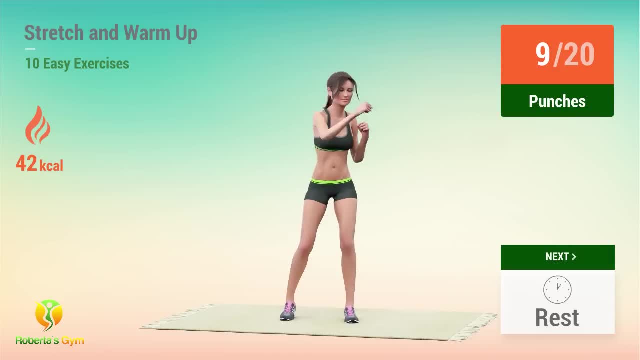 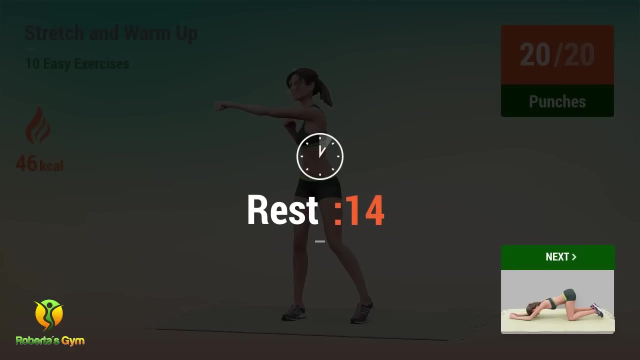 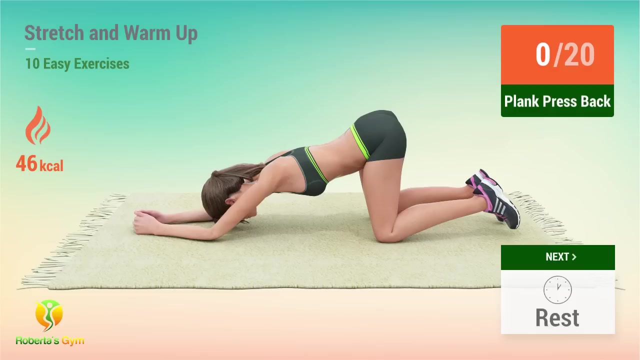 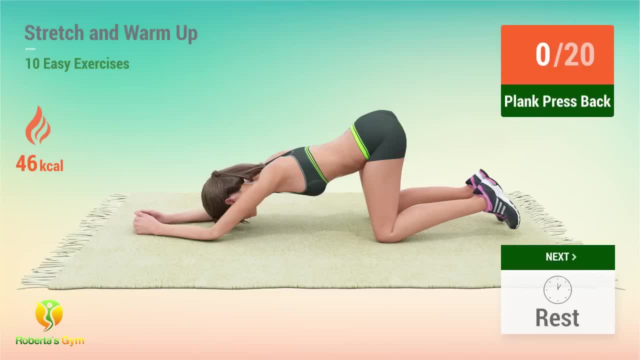 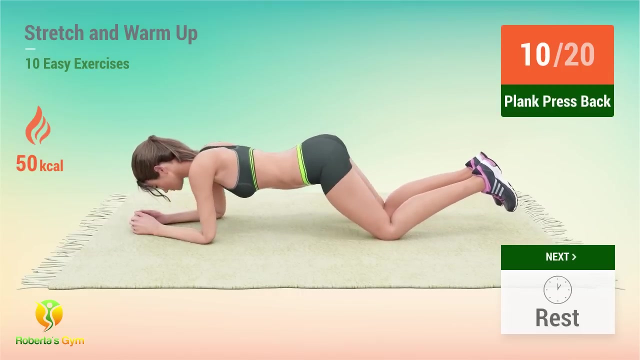 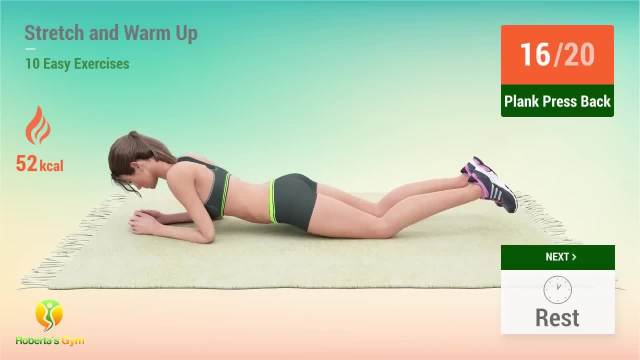 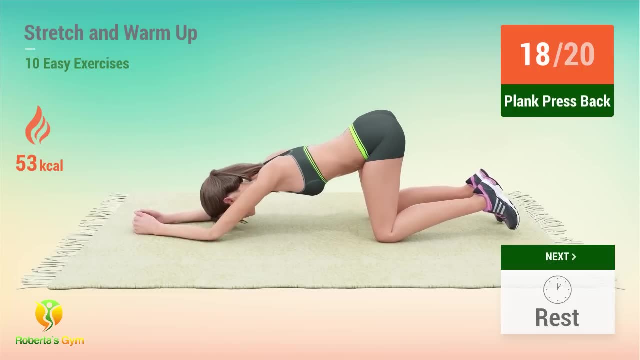 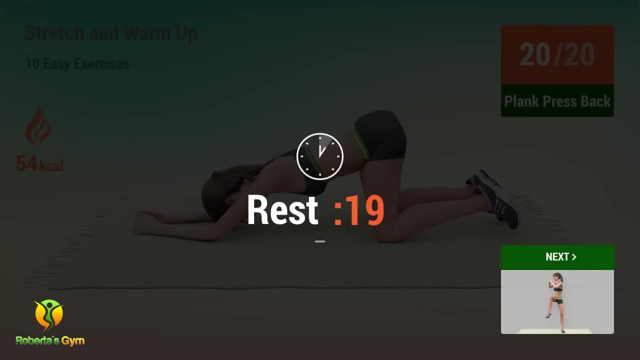 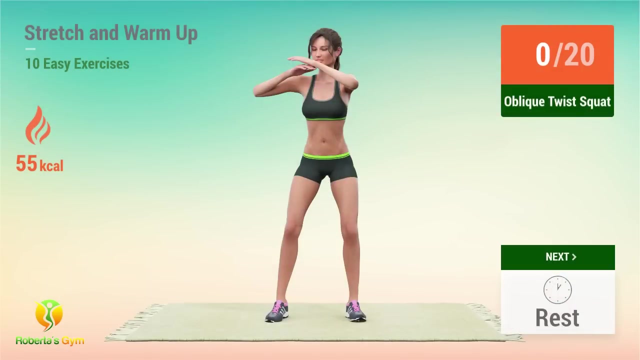 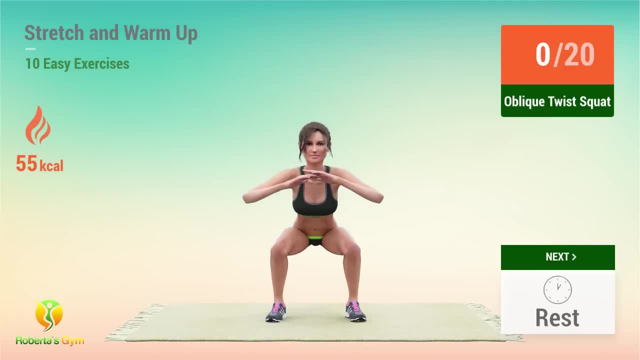 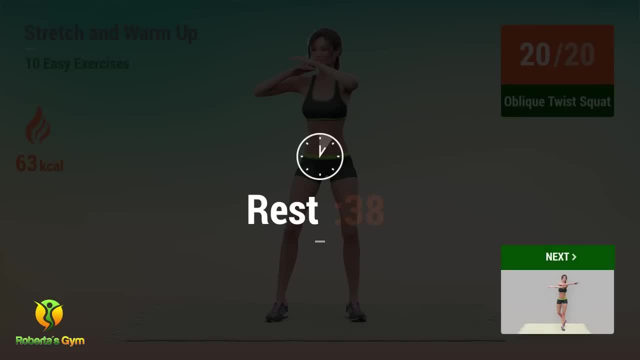 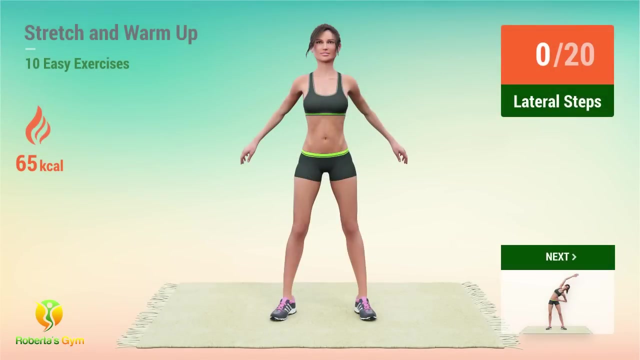 Rest time. Up next lateral steps In 5,, 4,, 3,, 2, 1, go 1,, 2,, 3,, 4, 5. Rest time 6,, 7,, 8,, 9,, 10,, 11,, 12,, 13,, 14,, 15,, 16,, 17,, 18,, 19, 20. 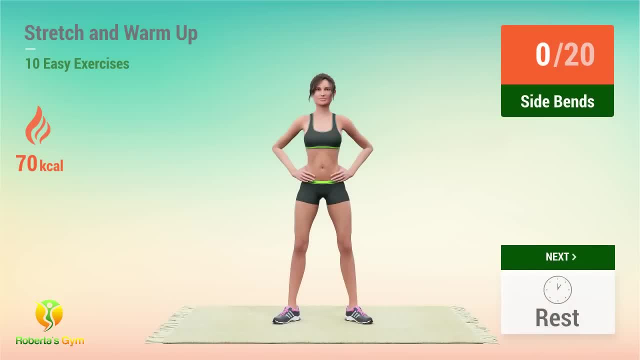 Up next side bends In 5,, 4,, 3,, 2,, 1, go 1,, 2,, 3,, 4,, 5,, 6,, 7,, 8,, 9,, 10,, 11,, 12,, 13,, 14,, 15,, 16,, 17,, 18,, 19,, 20. 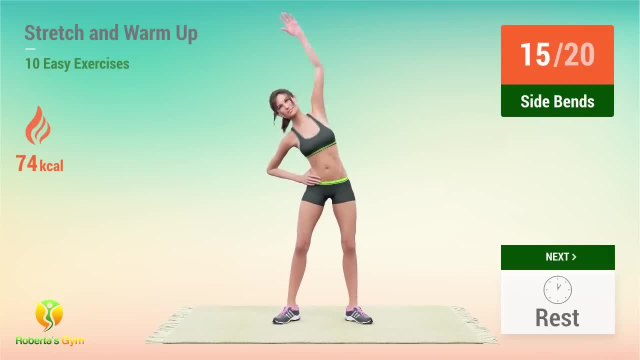 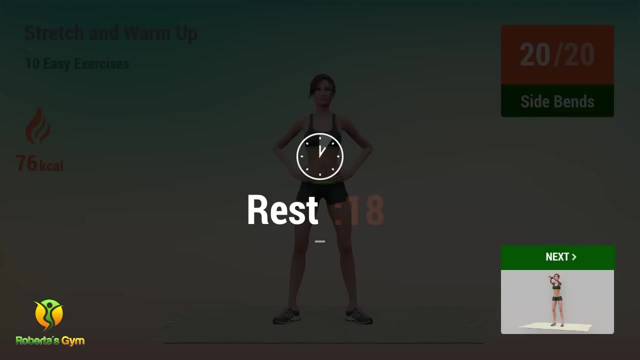 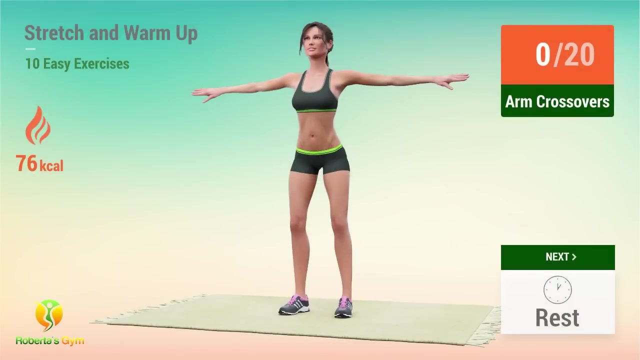 14,, 15,, 16,, 17,, 18,, 19, 20. Rest time Up next arm crossovers In 5,, 4,, 3,, 2, 1, go 1,, 2,, 3,, 4,, 5,, 6,, 7,, 8,, 9,, 10,, 11,, 12,, 13,, 18,, 19,, 20. 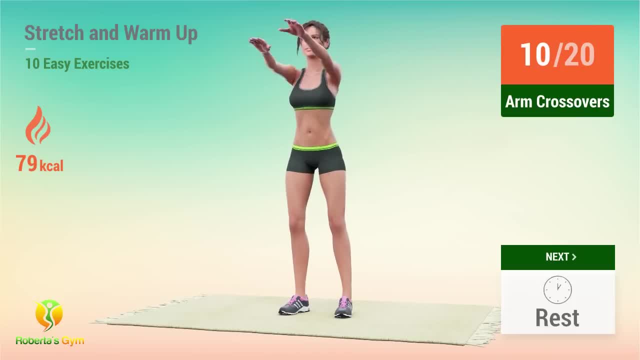 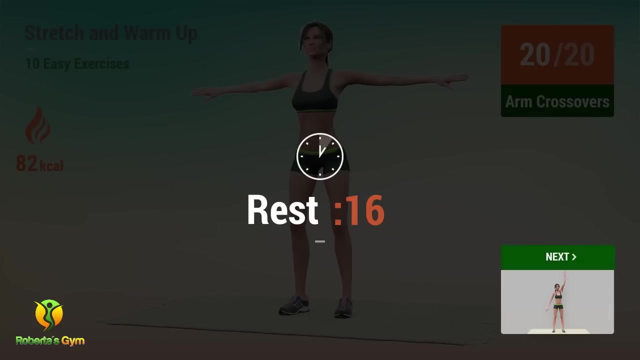 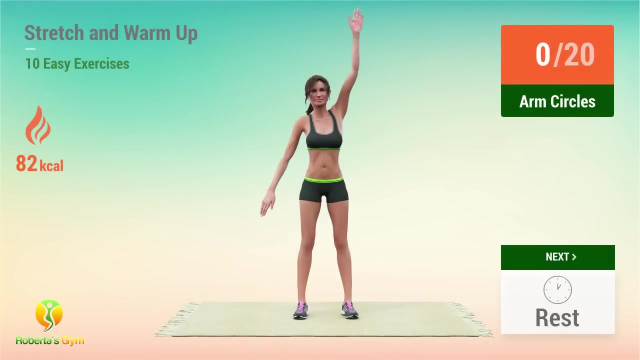 9, 10, 11, 12, 13, 14, 15, 16, 17, 18, 19, 20. Rest Time: 15, 16, 17, 18, 19, 20, 21, 22, 23, 24, 25, 26, 27. 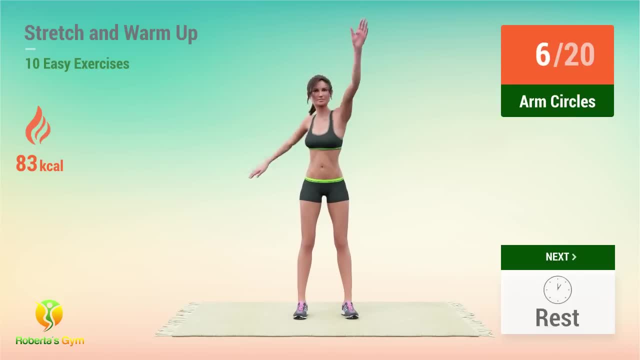 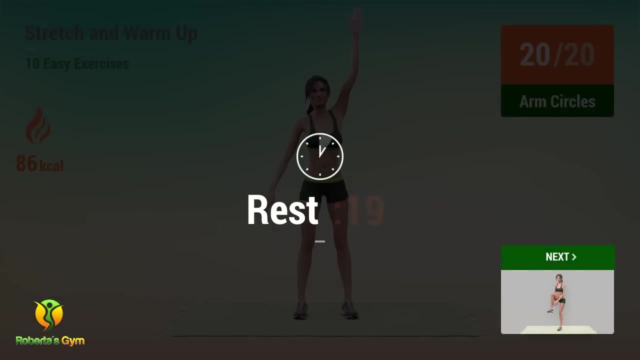 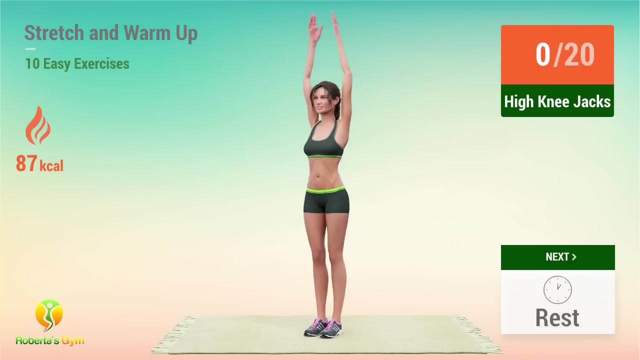 28, 29, 30, 31, 32, 33, 34, 35, 36, 37, 38, 39, 40, 41, 42, 43, 44, 45, 46, 47, 48, 49, 50, 51, 52, 53. 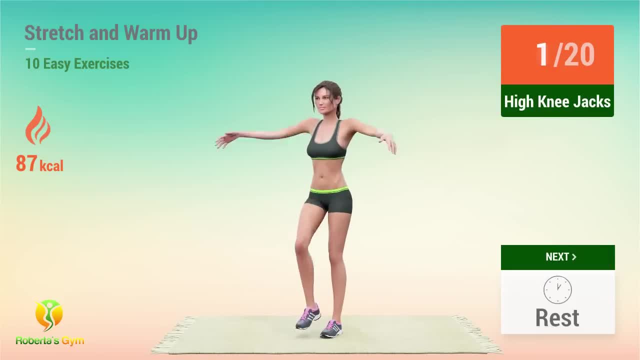 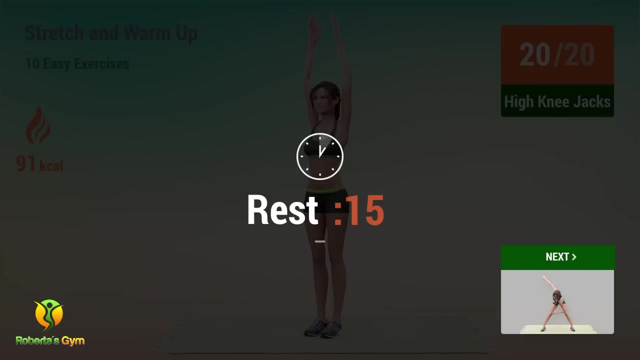 54, 55, 56, 57, 58, 59, 59, 60, 61, 62, 63, 64, 65, 66, 67, 68, 69, 70, 71, 72, 73, 74, 75, 76, 77, 78. 79, 80, 81, 82, 83, 83, 84, 85, 86, 87, 88, 89, 90, 91, 92, 93, 94, 95, 96, 97, 97, 98, 99, 100, 100, 100. 0, 7, 8, 3, 4, 3, 1, 1, 3, 9, 10, 4, 5, 6, 7, 6, 9, 10, 7, 8, 9, 10, 11, 12, 13, 14. 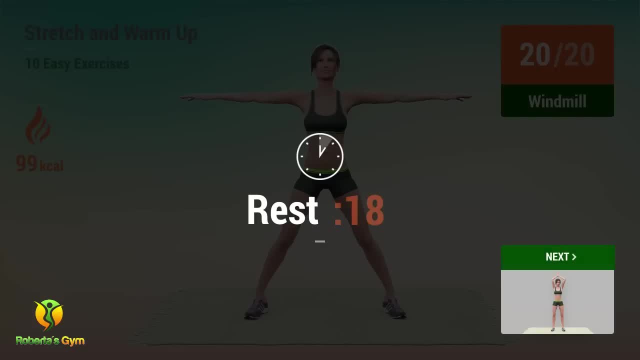 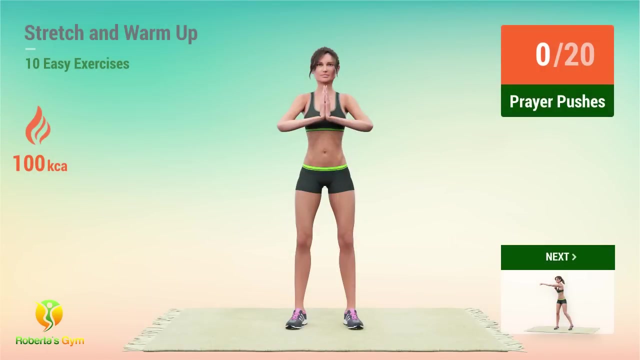 15, 65 Next time Up. next prayer pushes In five, four, three, two, one go One, two, three, four, five, six, seven, eight, nine, 10,, 11,, 12,, 13,, 14,, 15,, 16,, 17,, 18,, 19,. 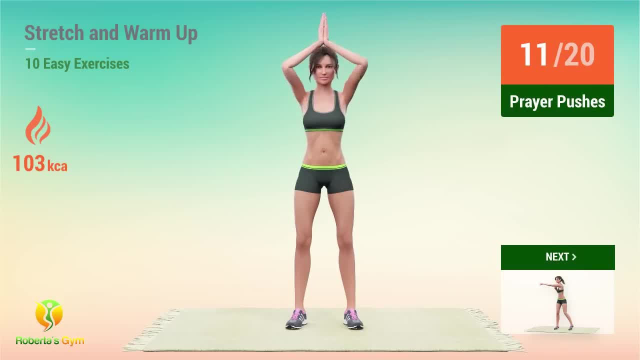 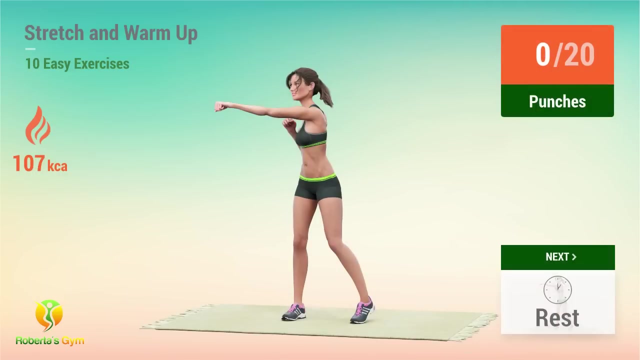 20.. Up next punches In five, four, three, two, one go. One, two, three, four, five, six, seven, 18,, 19,, 20.. Up next prayer punches: One, two, one go. 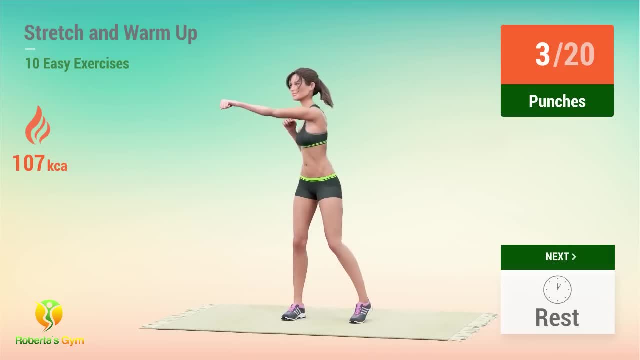 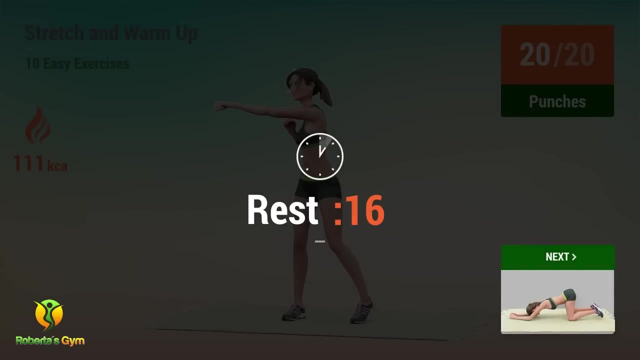 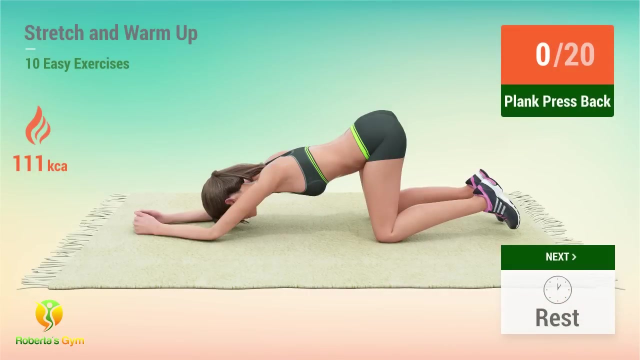 One, two, three, four, five, six, seven, eight, nine, ten, eleven, twelve, thirteen, fourteen, fifteen, sixteen, seventeen, eighteen, nineteen, twenty. Rest time Up next plank. press back in five, four, three, two, one go. 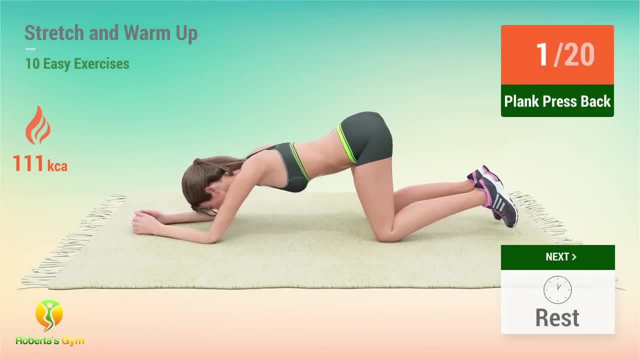 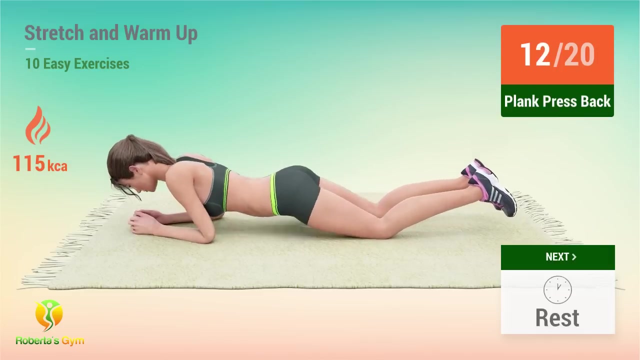 One, two, three, four, five, six, seven, eight, nine, ten, eleven, twelve, thirteen, eight, nine, ten, eleven, twelve, thirteen, fourteen, fifteen, sixteen, seventeen, eighteen, nineteen, twenty. 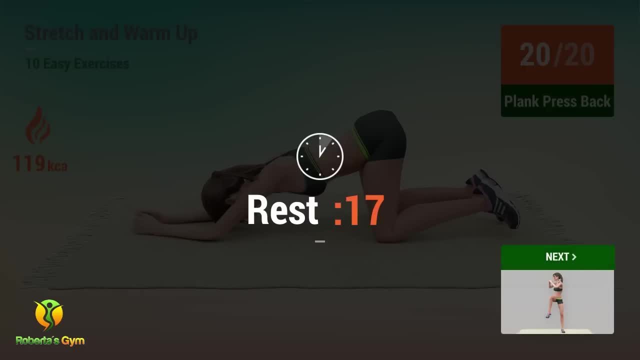 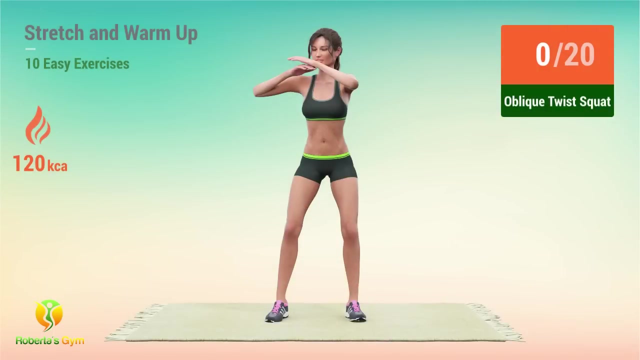 Rest time. Up next, oblique twist squat In five, Five, four, three, two. one go One, two, three, four, five, six, seven, eight, nine, ten, eleven, twelve, thirteen. 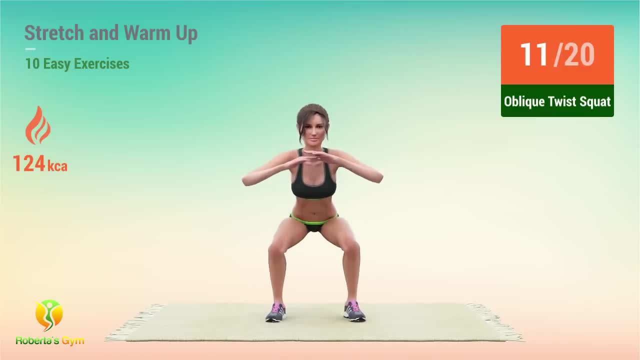 eleven, twelve, thirteen, fourteen, fifteen, sixteen, seventeen, eighteen, nineteen, twenty Rest time Up next plank. press back in: five, four, three, two, one go. One, two, three, two, one go. 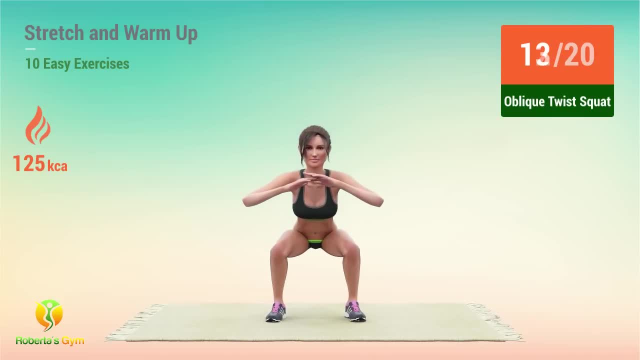 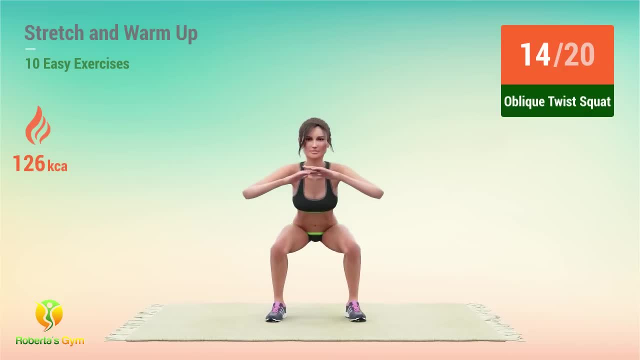 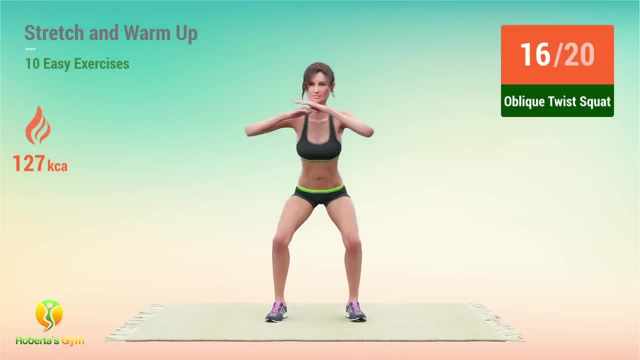 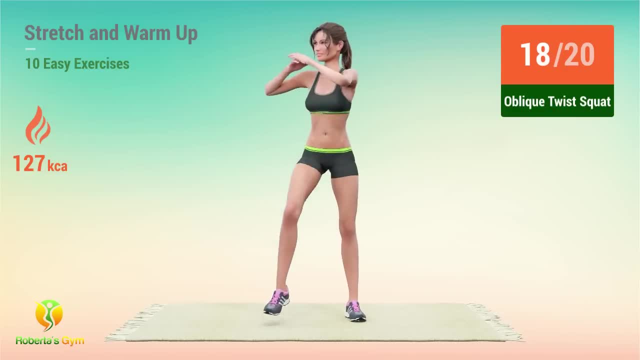 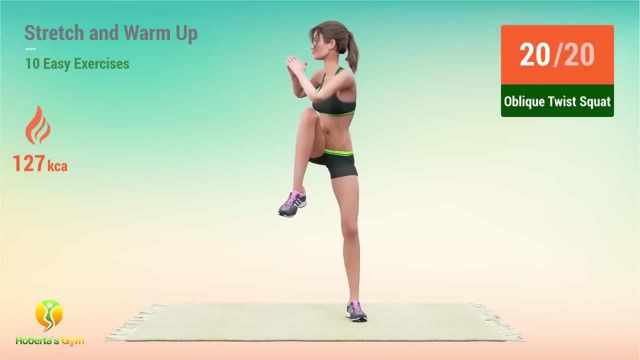 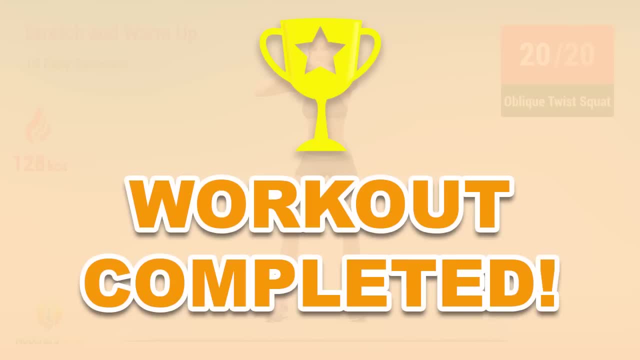 One, two, three, two, one go. One, two, three, two, one go.